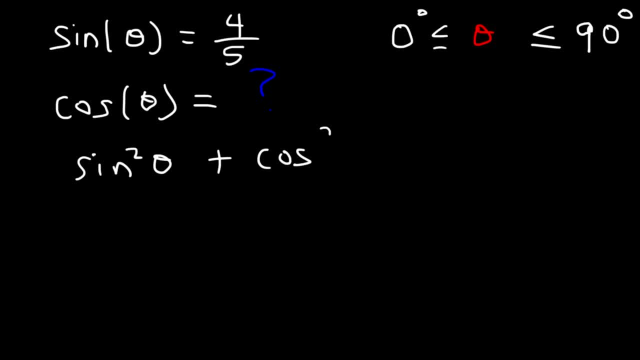 identity. sine squared plus cosine squared is 1.. If we know the value of sine, we can find the value of cosine Sine is 4 over 5.. So now let's calculate the value of cosine. 4 squared is 16.. 5 squared is 25.. And 1, we 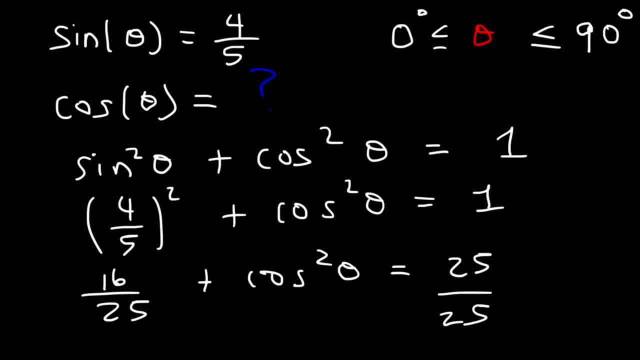 can write it as 25 divided by 25.. Now the next thing that we could do is we could subtract both sides by 16 over 25.. So, cosine squared, theta is 25 over 25 minus 16 over 25.. So that's. 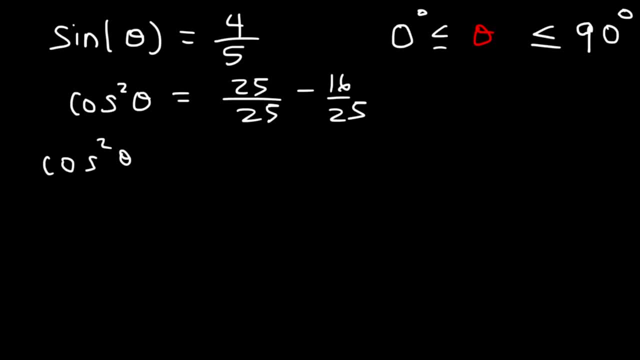 25.. 25 minus 16 is 9.. So we have 9 over 25.. And now we need to take the square root of both sides. The square root of 9 is 3.. The square root of 25 is 5.. Now it can be plus. 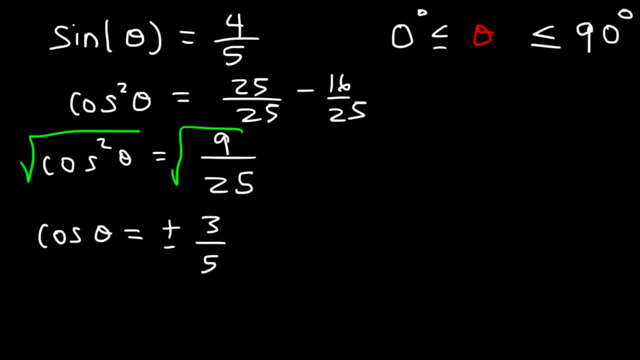 or minus 3 over 5.. Now, which sine should we choose? Should we choose positive 3 divided by 5 or negative 3 divided by 5?? To answer that question, we need to look at the angles. Theta is in quadrant one. It's between 0 and 90 degrees And in quadrant 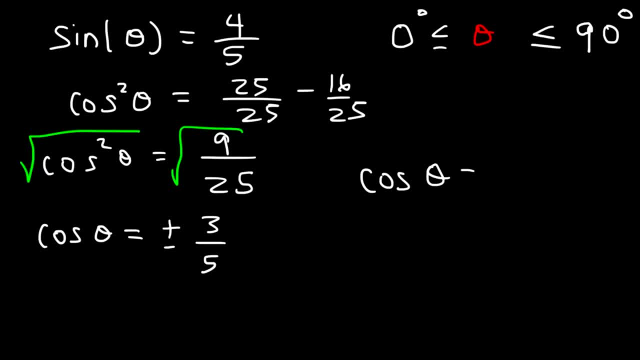 one cosine is positive. So the answer that we're going to have to choose is positive, 3 over 5.. So we need to use the quadrant to find the final sine. Let's try another example. Let's say cosine is equal to 8 over 17.. And let's say the angle. 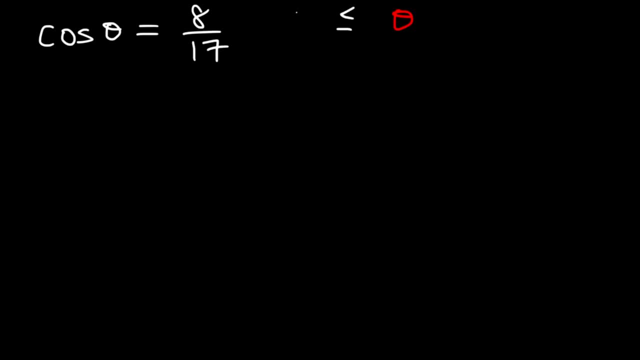 theta is 8 over 17.. between 3 pi over 2 and 2 pi. So, based on this, what is the value of sine? So let's use the same formula: Sine squared plus cosine squared is equal to 1.. So we need to find: 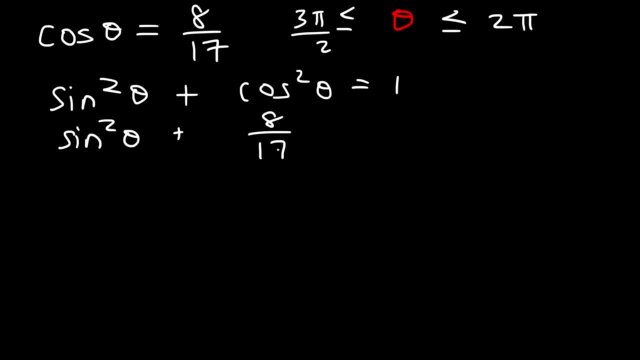 the value of sine Cosine is 8 over 17.. 8 squared is 64.. And 17 squared is 289.. And 1,. let's rewrite it as 289 divided by 289.. Any number divided by itself is 1.. So we got. 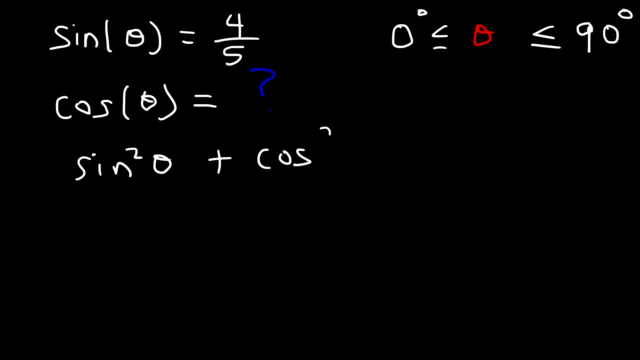 identity. sine squared plus cosine squared is 1.. If we know the value of sine, we can find the value of cosine Sine is 4 over 5.. So now let's calculate the value of cosine. 4 squared is 16.. 5 squared is 25.. And 1, we 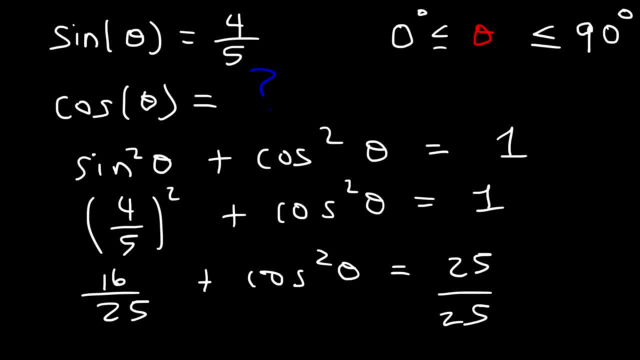 can write it as 25 divided by 25.. Now the next thing that we could do is we could subtract both sides by 16 over 25.. So, cosine squared, theta is 25 over 25 minus 16 over 25.. So that's. 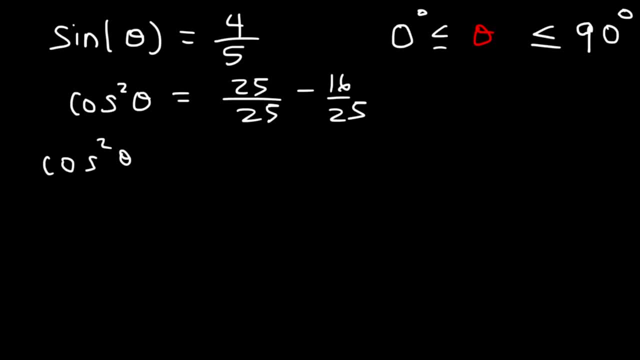 25.. 25 minus 16 is 9.. So we have 9 over 25.. And now we need to take the square root of both sides. The square root of 9 is 3.. The square root of 25 is 5.. Now it can be plus. 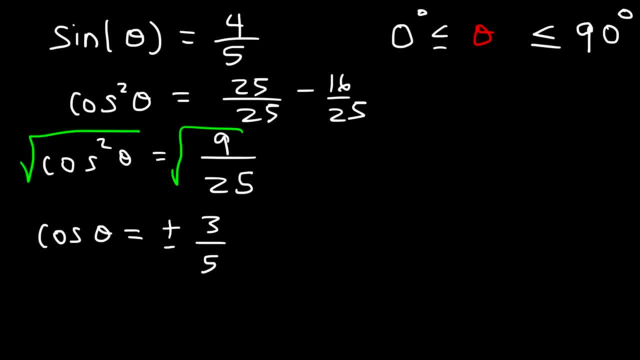 or minus 3 over 5.. Now, which sine should we choose? Should we choose positive 3 divided by 5 or negative 3 divided by 5?? To answer that question, we need to look at the angles. Theta is in quadrant 1.. It's between 0 and 90 degrees And in quadrant. 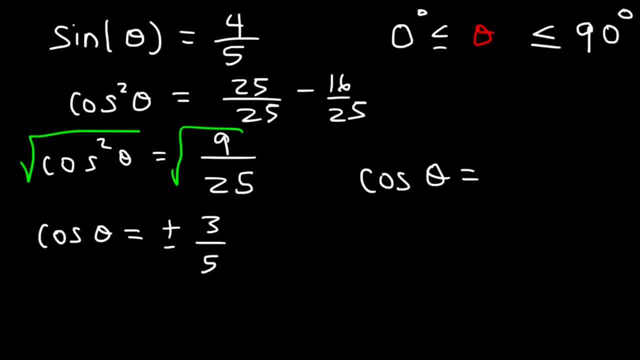 1, cosine is positive, So the answer that we're going to have to choose is positive, 3 over 5.. So we need to use the quadrant to find the final sine. Let's try another example. Let's say cosine is equal to 8 over 17.. And let's say the angle. 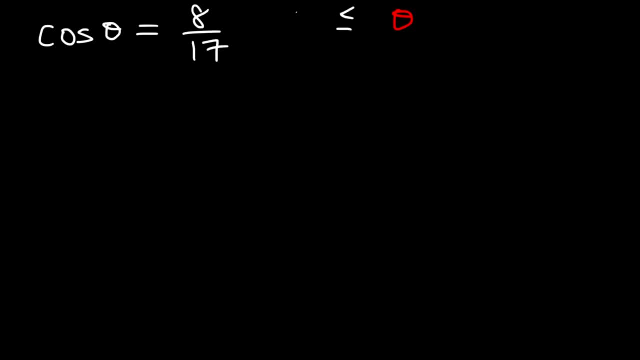 theta is 0 over 5.. It's between 3 pi over 2 and 2 pi. So, based on this, what is the value of sine? So let's use the same formula: Sine squared plus cosine squared is equal to 1.. So we need to find: 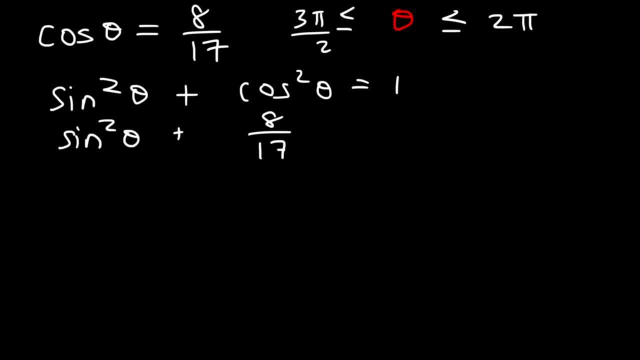 the value of sine Cosine is 8 over 17.. 8 squared is 64. And 17 squared is 289.. And 1,. let's rewrite it as 289 divided by 289.. Any number divided by itself is 1.. So we got to subtract 289 by 64. So sine squared is equal to 225 divided. 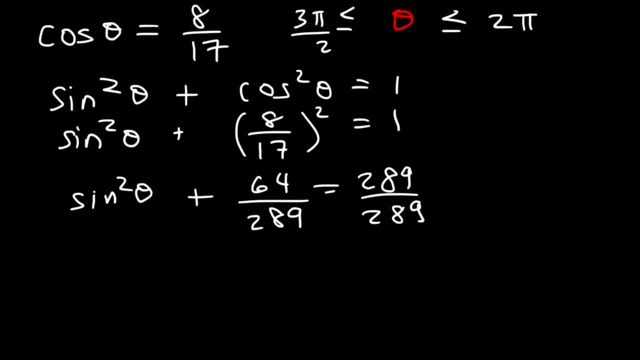 to subtract 289 by 64.. So sine squared is equal to 225 divided by 289.. Now let's take the square root of both sides. So sine theta is going to be: the square root of 225 is 15.. And we know the square root of 289 is 17.. 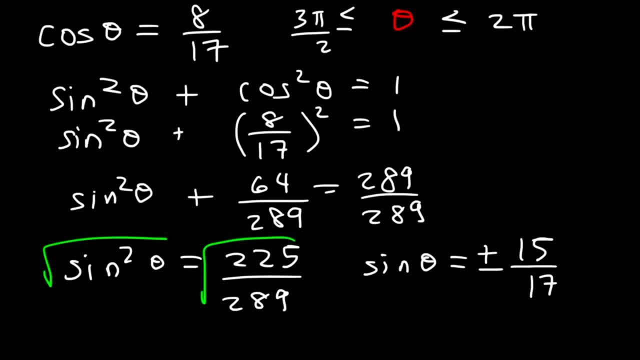 So now, which sine should we use, Positive or negative? So if the angle is between 3 pi over 2 and 2 pi, what quadrant is it located in? Now, keep in mind, 3 pi over 2 is equivalent to 270.. 2 pi is 360.. So 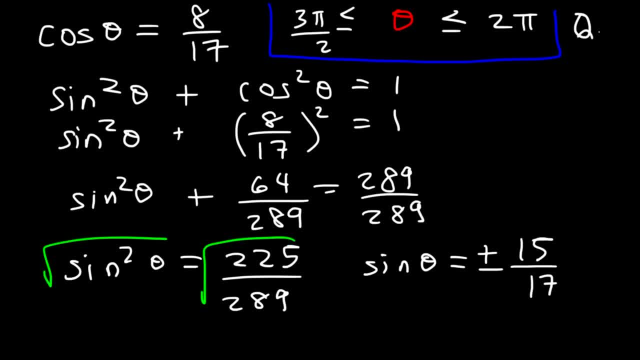 it's located in quadrant 4.. And in quadrant 4, sine is negative, but cosine is positive. So therefore, sine is going to be negative 15 over 17 in this particular example, And so that's the answer. Let's try one more example. Let's say that sine is negative 15 over 17.. 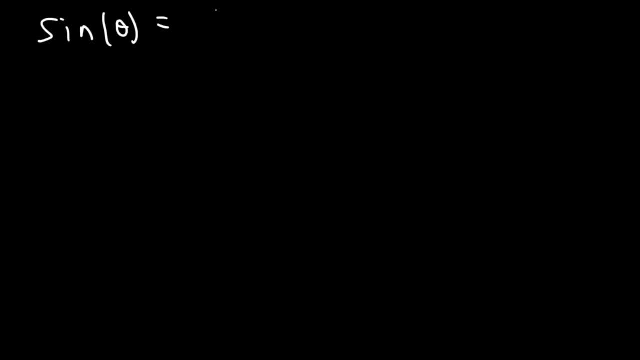 that sine theta is equal to 2 over 5 and tangent theta is less than 0. What is the value of cosine theta? So before we use the formula, let's find out what quadrant the angle is located in. So first we know that sine is positive. Sine is positive in quadrants 1. 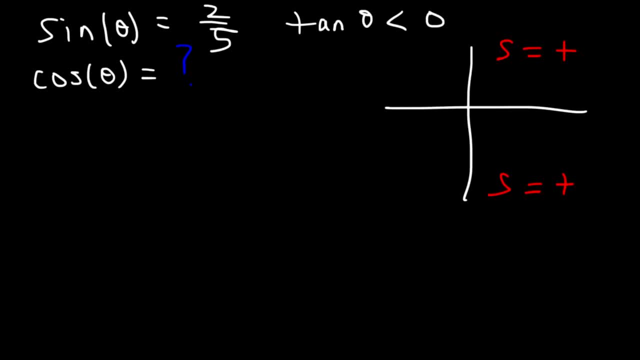 and 4.. Now tangent is less than 0.. Tangent is positive in quadrants 1 and 3. Tangent is y over x In quadrant 1, x and y are both positive. So if you divide a positive number, 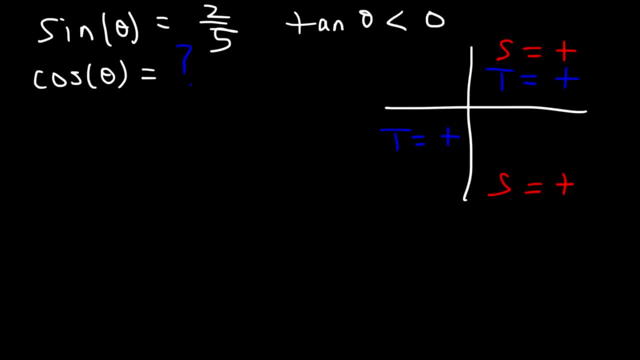 by a positive number, it's going to be positive In quadrant 3, x and y are both negative. When you divide two negative numbers, you'll get a positive value In quadrants 2 and 4, tangent is negative. Now we know tangent is. 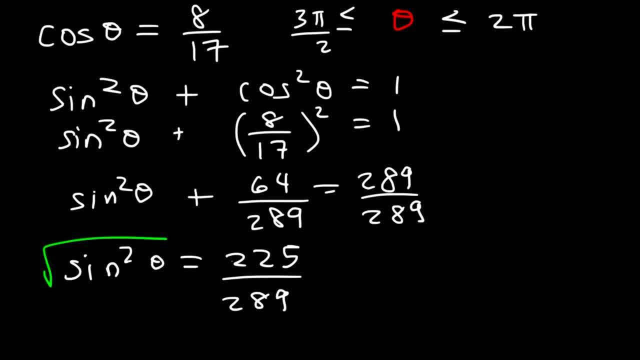 by 289.. Now let's take the square root of both sides. So sine theta is going to be: the square root of 225 is 15.. And we know the square root of 289 is 17.. So now, which sine should we use? Positive or negative? 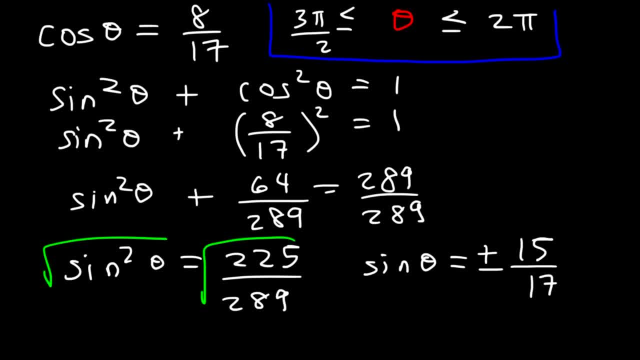 So if the angle is between 3 pi over 2 and 2 pi, what quadrant is it located in? Now, keep in mind: 3 pi over 2 is equivalent to 270.. 2 pi is 360.. in quadrant 4.. And in quadrant 4, sine is negative but cosine is positive. So 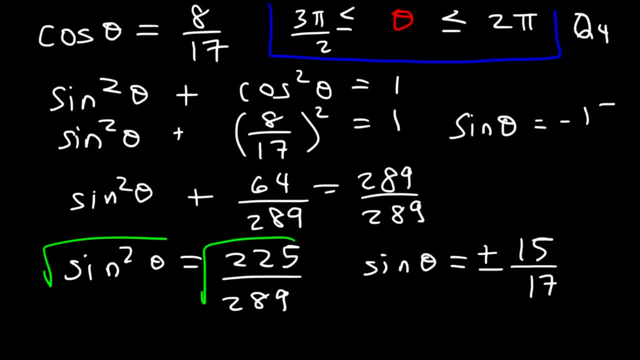 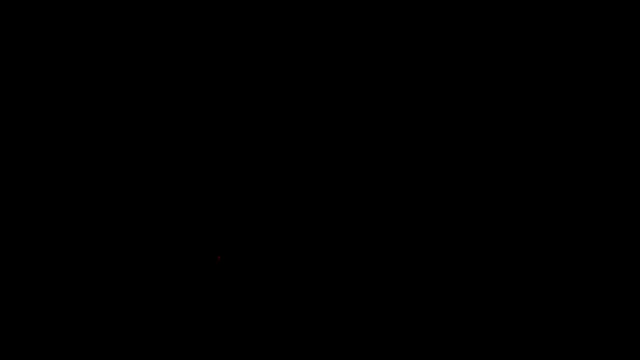 therefore, sine is going to be negative- 15 over 17 in this particular example- And so that's the answer. Let's try one more example. Let's say that sine theta is equal to 2 over 5, and tangent theta is less than 0. What is the value of cosine theta? 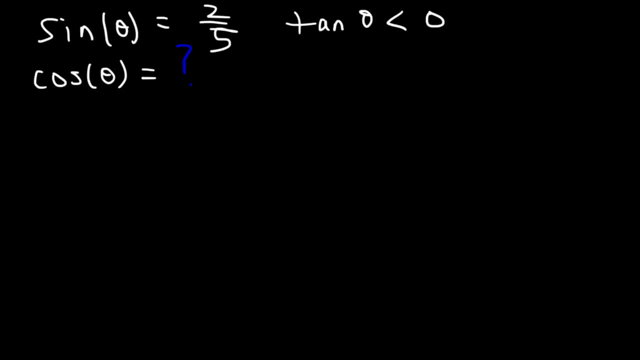 So before we use the formula, let's find out what quadrant the angle is located in. So first we know that sine is positive. Sine is positive in quadrant 1, and sine is positive in quadrant 2.. Now tangent is less than 0.. Tangent is positive in quadrants 1 and 3.. 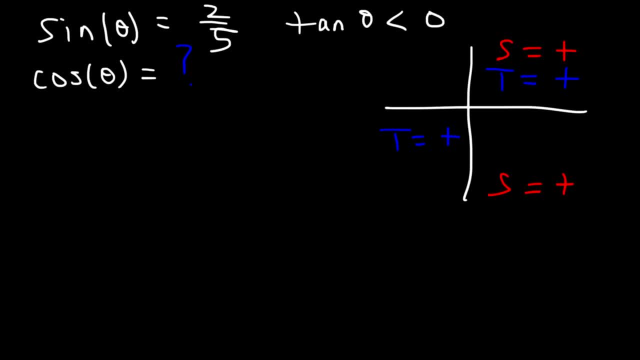 Tangent is y over x. In quadrant 1, x and y are both positive. So if you divide a positive number by a positive number, it's going to be positive. In quadrant 3, x and y are both negative. When you divide two negative numbers, you'll get a positive value. 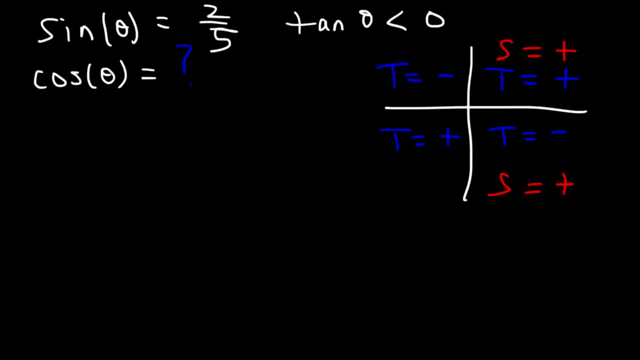 In quadrants 2 and 4, sine is positive, Tangent is negative. Now we know tangent is less than 0. So it's less than 0 or negative in quadrants 2 and 4.. But sine has to be positive. So both statements are true in. 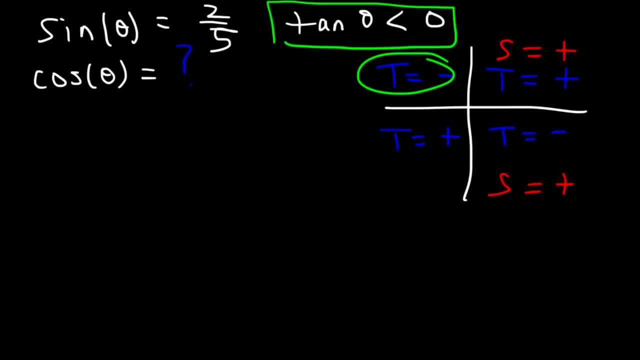 quadrant 4.. Sine is positive, but tangent is negative. Now cosine is positive. Cosine is positive In quadrants 1 and 4.. Since our angle is in quadrant 4, we know our final answer has to be positive. So just keep that in mind.